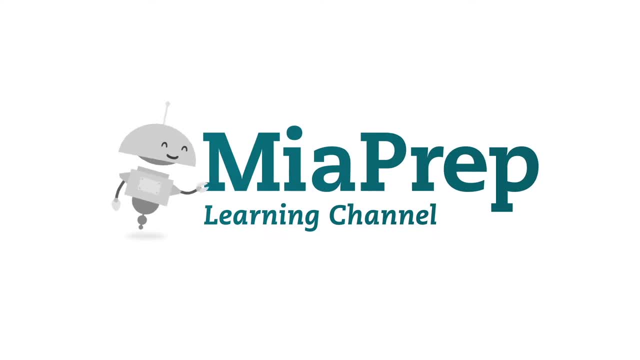 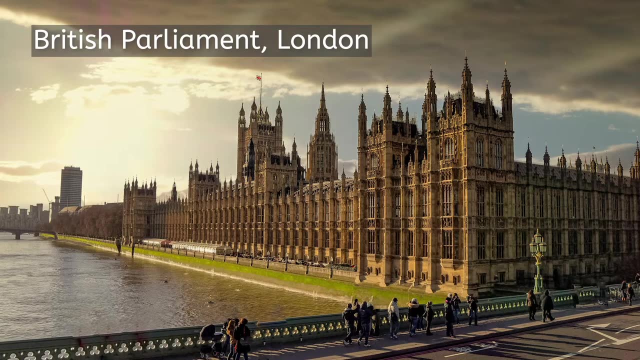 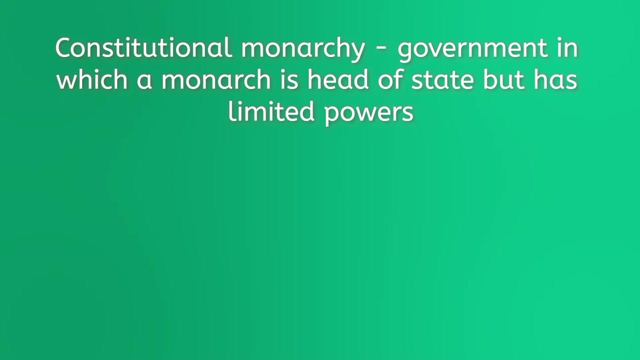 Government. So first of all, let's look at the political structures of these five nations. You may be especially surprised at this first nugget of information. Did you know that four of these five nations are constitutional monarchies? It's true, In a constitutional monarchy. 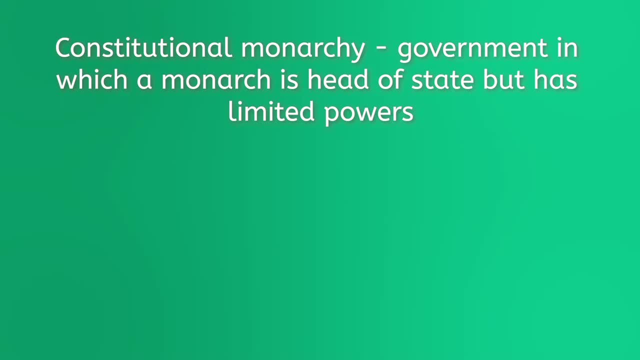 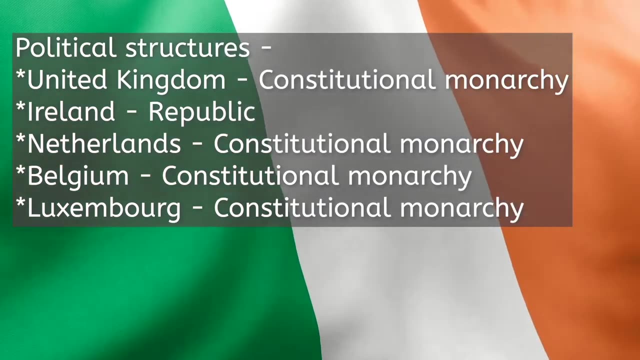 the person in charge has a title such as king, queen or duke. In this region, Ireland is unique in that its government is a republic. The other nations are all constitutional monarchies, Though they have elected leaders, such as prime ministers, to handle most political affairs. 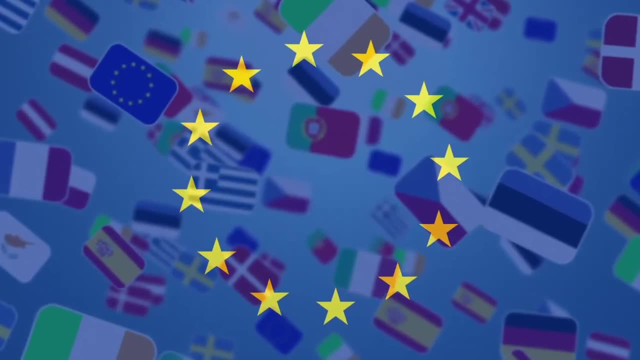 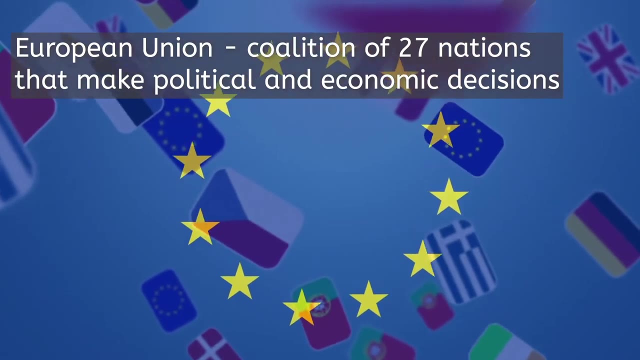 all are officially led by royalty. Next, you've heard us reference the European Union several times. 1. The European Union is a coalition of 27 nations. The European Union is a coalition of 27 nations on the continent that make political and economic decisions for the 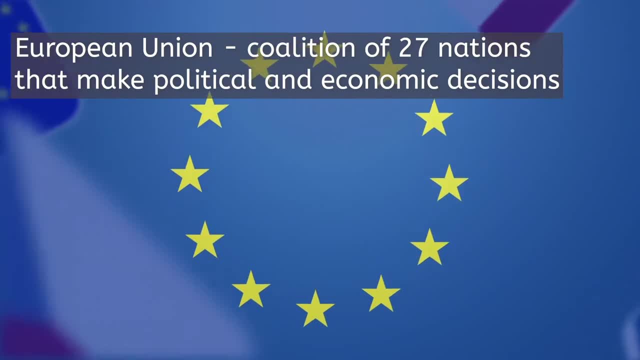 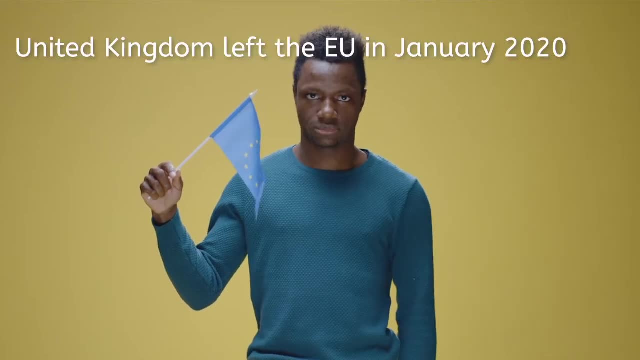 betterment of Europe. Did you know that only four of the five nations in Western Europe are members? It's a fact: In the United Kingdom, a former member of the EU actually dropped out of the alliance in January 2020.. Meanwhile, Ireland, Luxembourg, Belgium and the Netherlands. 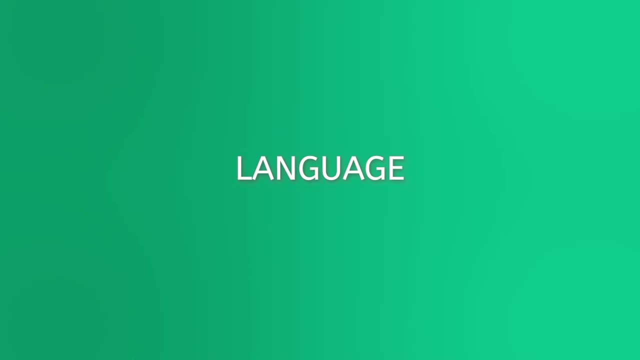 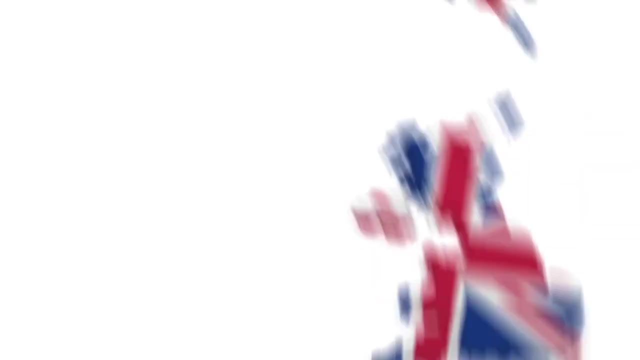 all remain members of the EU. 2. Language: Now, you might think that all of these nations speak English, And if so you'd be mistaken. The United Kingdom of Great Britain and Northern Ireland does in fact speak English, Although 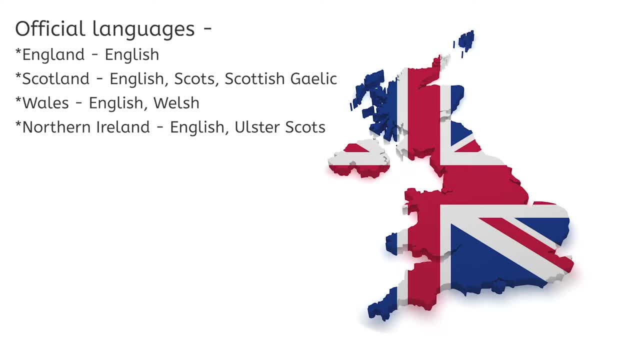 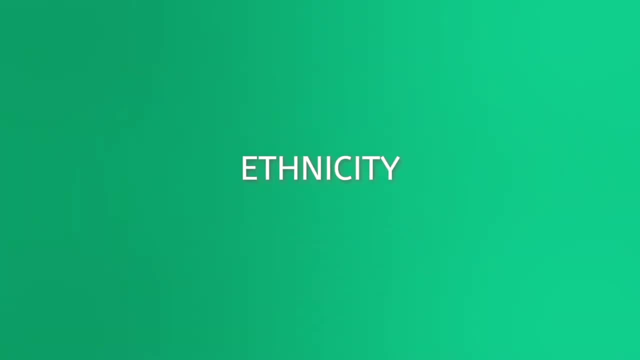 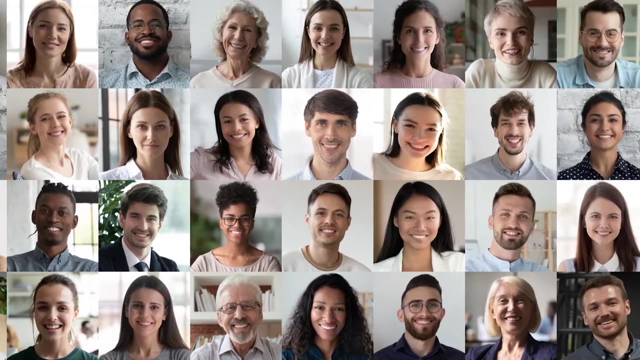 each nation of the Kingdom other than England employs other languages as well. Ireland is the only other nation in which English is an official language. 3. Ethnicity: When looking at this data, keep in mind that each nation selects its own criteria when identifying ethnicity. a nuance seen in Latin. 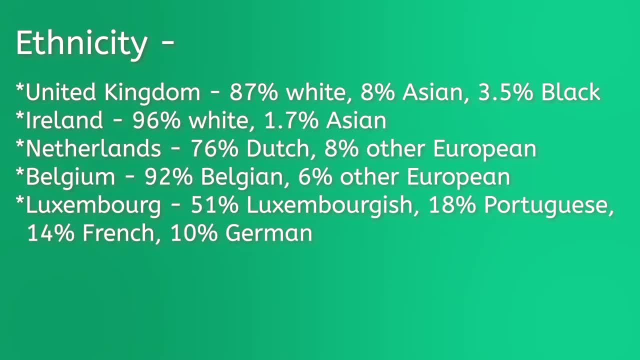 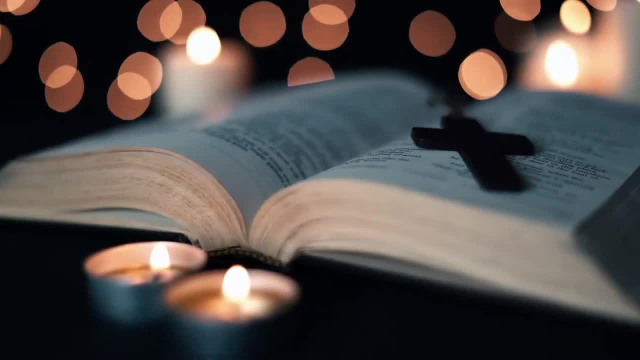 America as well. The populations in each nation vary, but are predominantly European. For example, England is the only country in the world that has an ethnic identity. and England is the only country in the world that has an ethnic identity. 4. Religion: You'd expect Europe to be largely Christian. 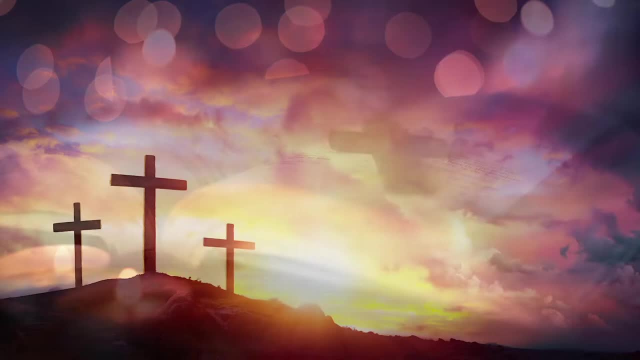 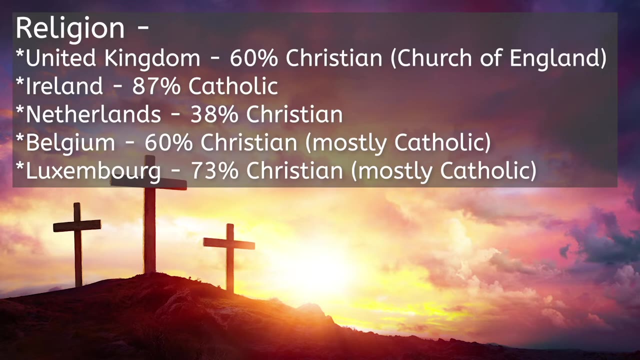 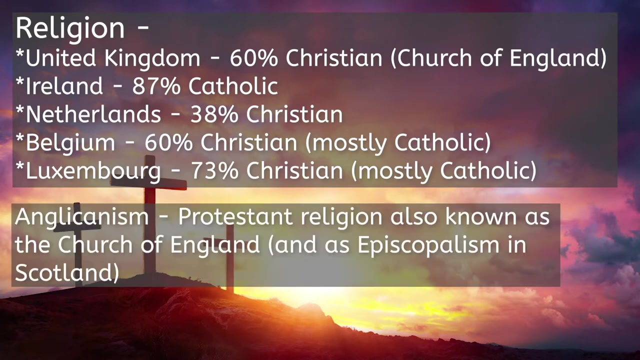 and this region certainly meets that expectation. But different forms of Christianity are preferred in different regions. The Republic of Ireland is overwhelmingly Catholic. Northern Ireland is not. Rather, it is mostly Protestant. Specifically, Northern Ireland adheres to beliefs from the Church of England or Anglicanism, which is referred to as Episcopalianism in Scotland. 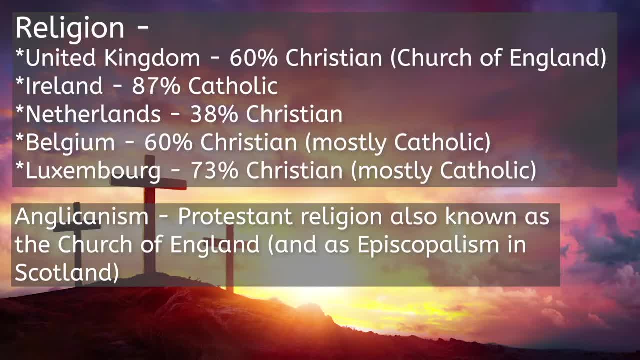 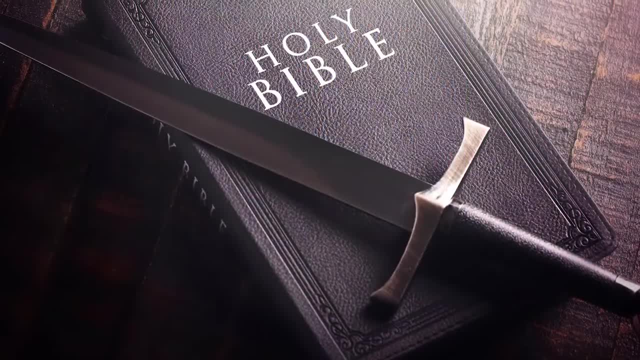 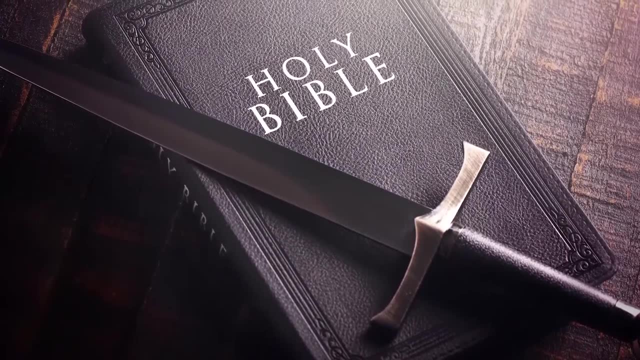 Both Belgium and Luxembourg, Catholicism is the religion of majority preference. Back to the religious diversions between Ireland and Northern Ireland, Those differences in beliefs are actually what precipitated the political division as well. The Home Rule Movement. Ireland's campaign for self-government culminated in 1922 with most of the island. 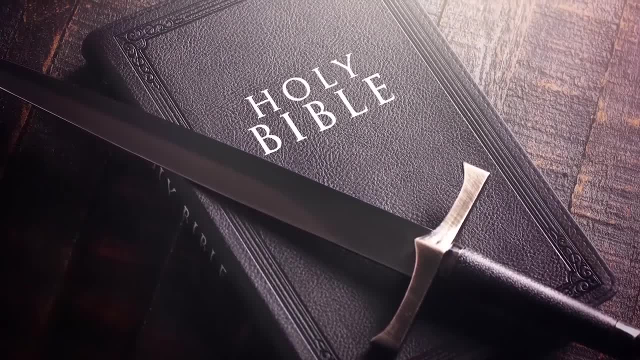 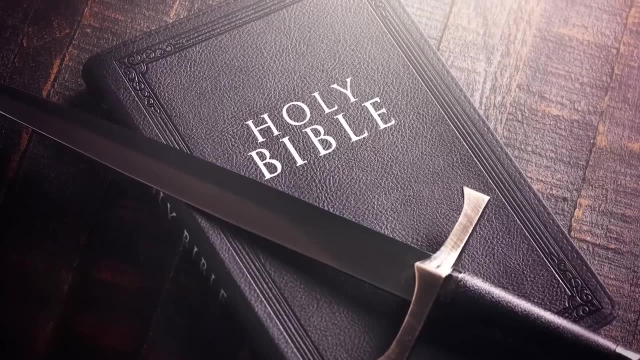 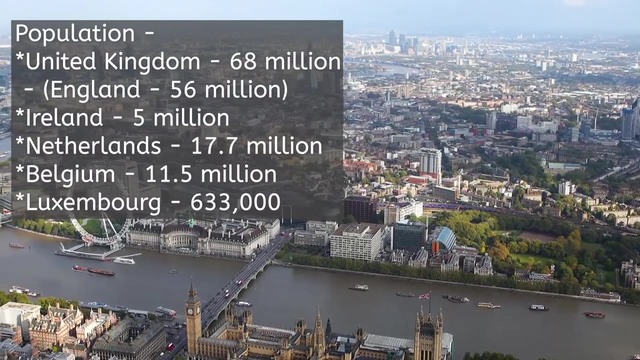 breaking free from Britain and forming the Irish Free State, which later evolved into the Republic of Ireland. The dispute lingered as violence was common on the island throughout the 20th century. 5. Population: The United Kingdom, with 68 million, is Europe's. 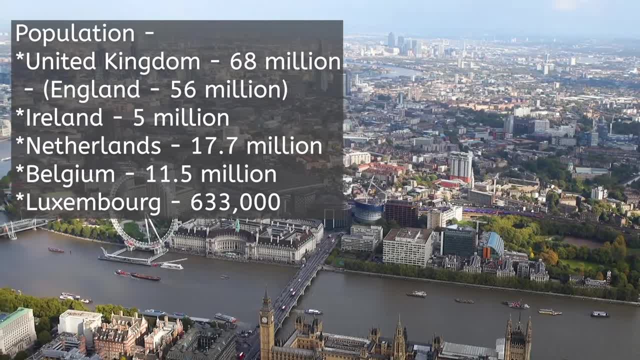 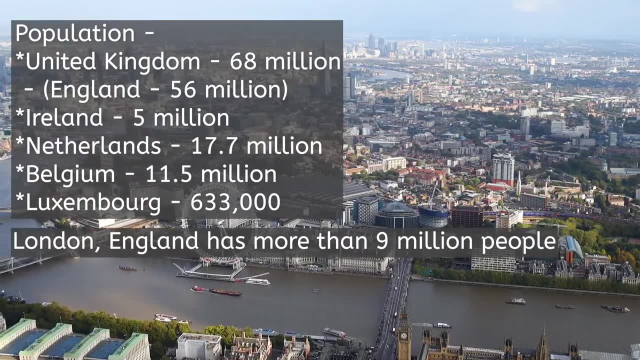 third-largest nation, behind only Russia and Germany. The bulk of those residents live in England. London, with more than 9 million people, is by far the largest city of the region. None of the other nations in the region surpass the Netherlands' 17.7 million as. 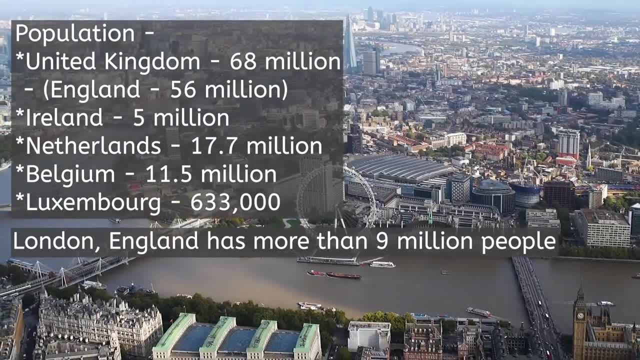 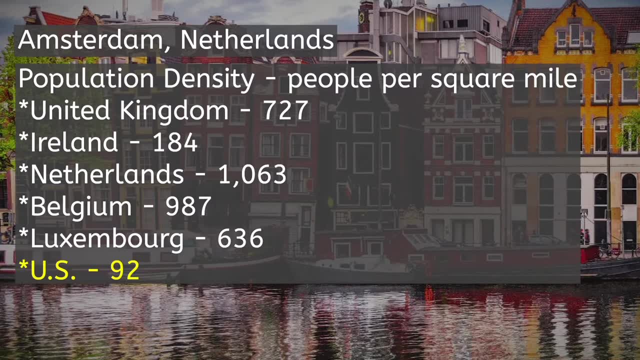 of 2021,, although that number is the tenth highest in Europe. 6. Population Density: Consider population density, however, to be different. The Netherlands has more than 1,000 people per square mile, the highest in Europe of any nation that is not a microstate such as Vatican City. Still, none of the citizens. 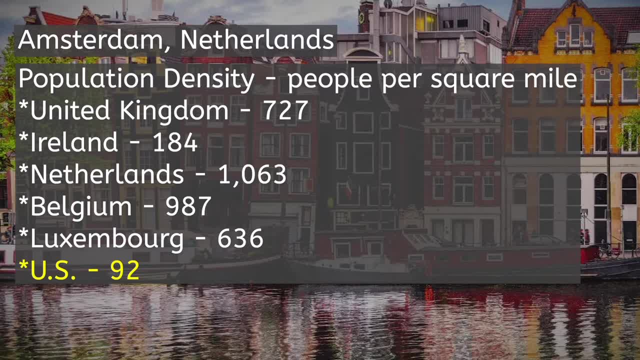 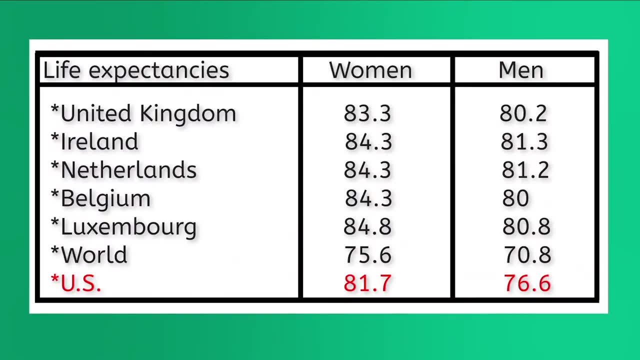 in these nations has the opportunity to find solitude in the wide-open spaces like we enjoy here in the US. On the other hand, perhaps having close neighbors is healthy. Each of these nations has life expectancies surpassing that of the United States, for both men and 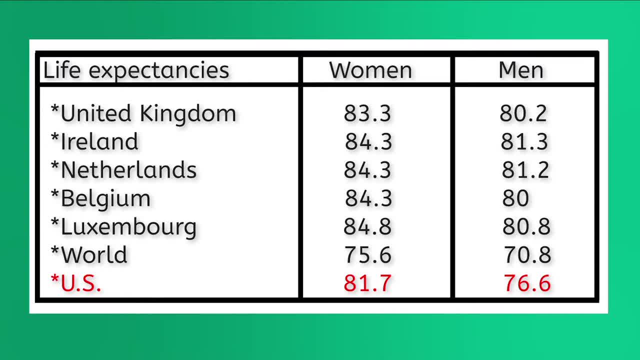 women. The US is significantly higher than the worldwide averages of 75.6 years for women and 70.8 years for men. Kinda makes you wonder what they're doing that we in the US aren't, huh? 7. Economies: No matter how you measure wealth, the five 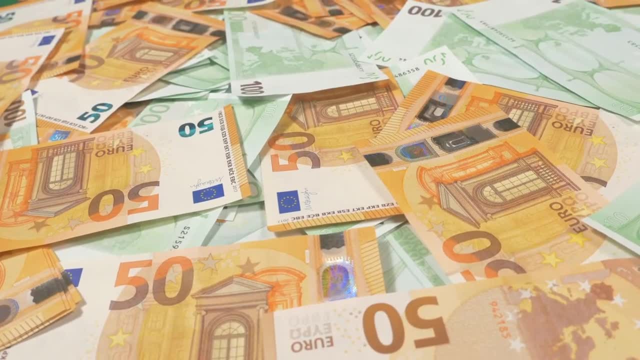 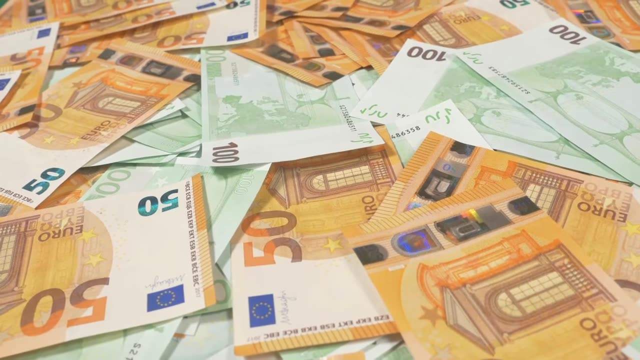 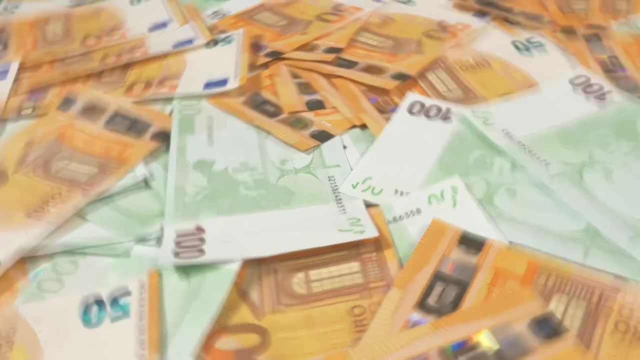 nations of Western Europe are among the most prosperous in the world. All are developed nations. All have transitioned from industrial to service-oriented economies, with large numbers of people working in tertiary activity professions. 7. Economic Efficiency. And all of these nations are ranked high on the Indices of Economic Freedom. 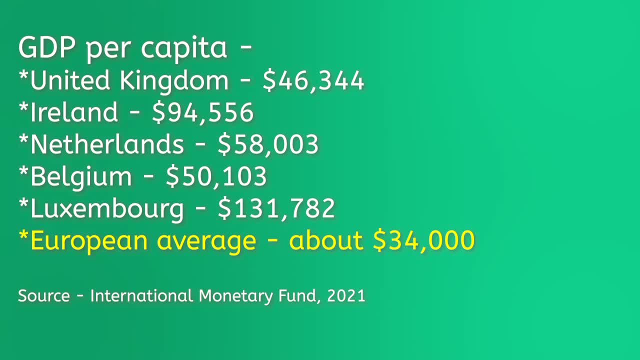 Take a look at each nation's estimated GDP per capita for 2021, as provided by the International Monetary Fund. The UK, though 29th in the world, actually lags behind its Western European neighbors, though all are well above the European average. Of special interest is Luxembourg. 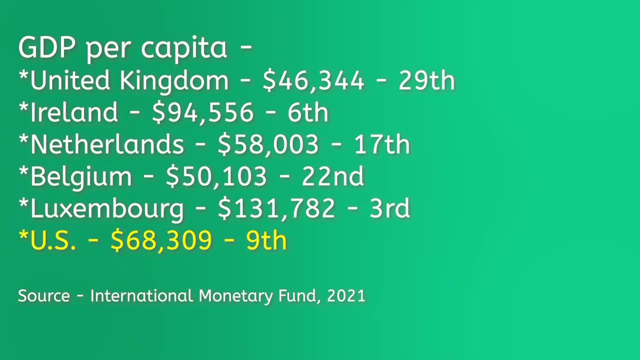 with the third highest GDP per capita in the world, and Ireland with the sixth highest. Both are ranked higher than even the United States. 8. GDP per capita in the world and the UK are ranked higher than even the United States. 9. GDP per capita in the world and the UK are ranked higher than even the United States. 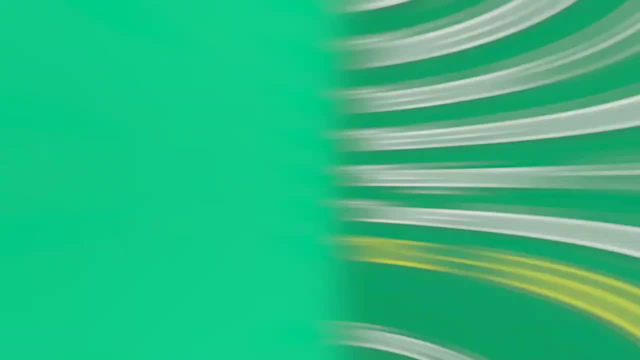 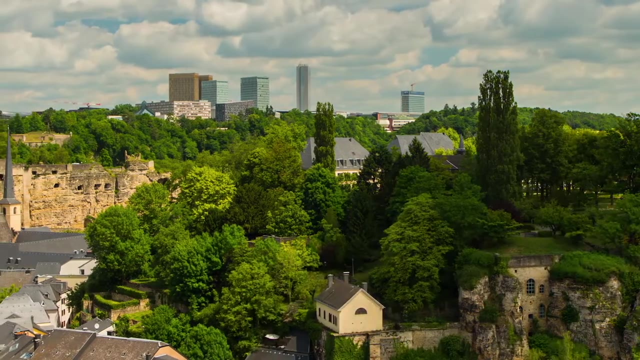 10. GDP per capita in the world, and the UK are ranked higher than even the United States. So what makes these nations so successful? Let's start with Luxembourg. The industrial sector, once dominated by steel, has diversified to include rubber and chemicals. Growth in the financial sector over the last half century. 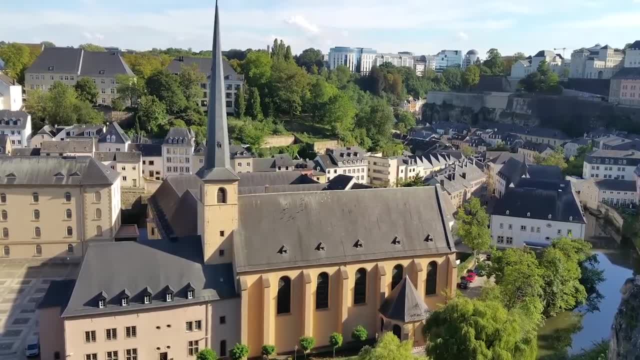 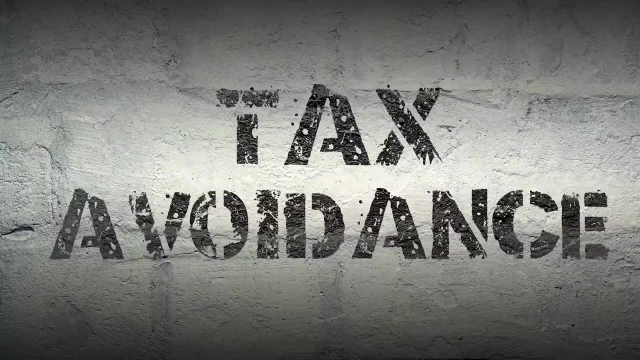 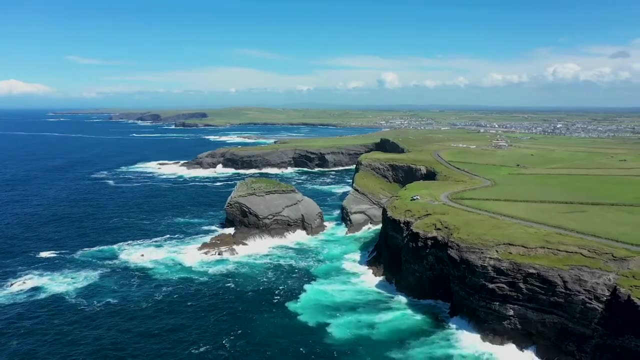 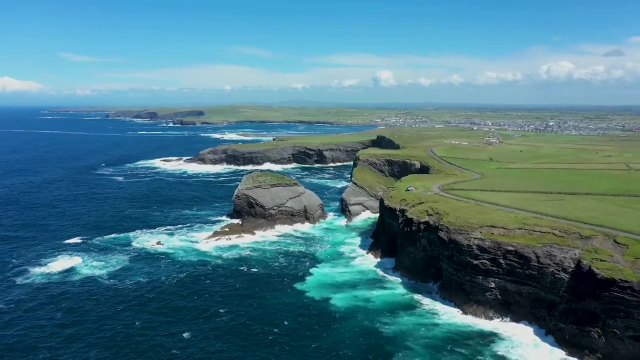 has propelled Luxembourg's economic rise, as services such as banking and investments account for most economic output. now, However, questions about banking practices and tax avoidance have plagued the nation since 2009.. Ireland features a service-oriented industry propelled by foreign multinational corporations. Exports are largely centered on pharmaceuticals, medical devices and software-related items. 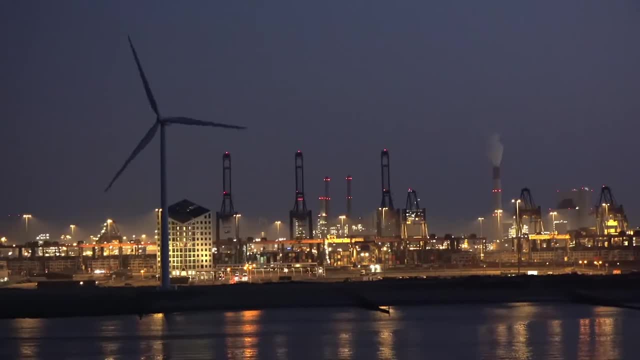 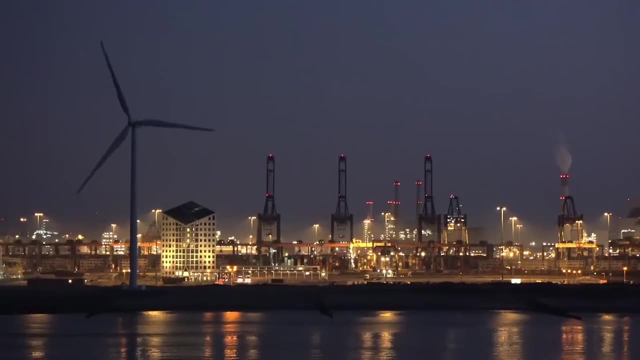 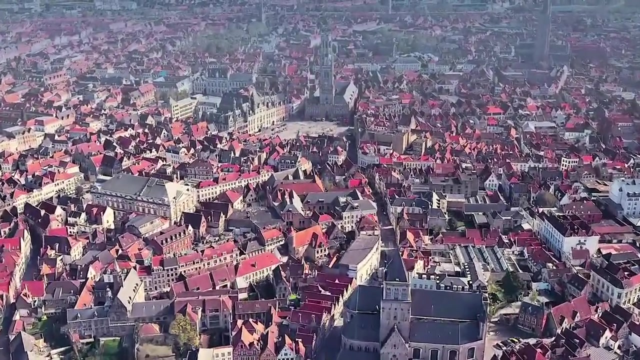 In the Netherlands. the port of Rotterdam is the largest in Europe and situated between prolific economies in Germany and the United Kingdom. Shipping is a major reason for financial success. Belgium's main exports are machinery and equipment, finished diamonds, chemicals, etc. Most work in a service profession, as Brussels is a highly industrialized center of employment. 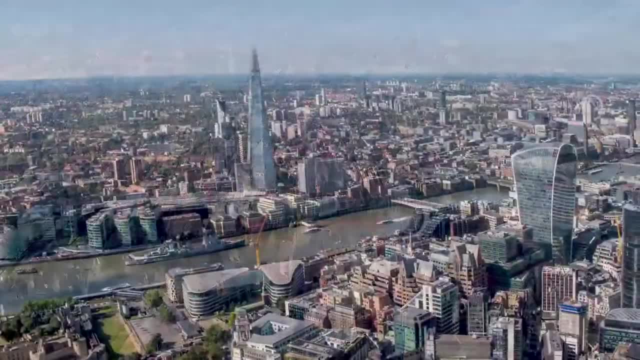 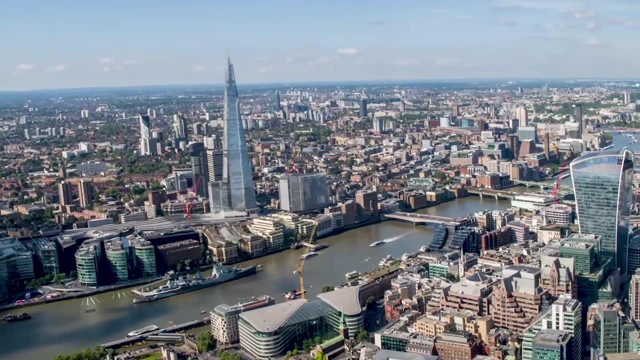 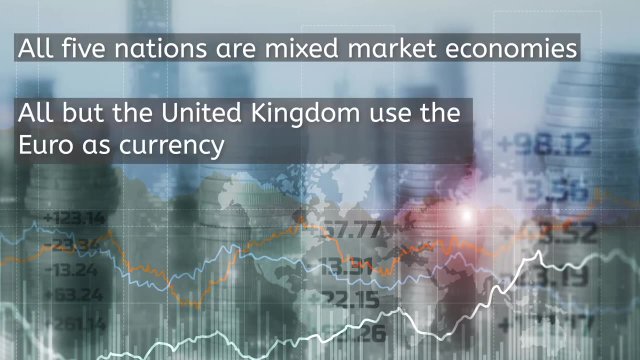 for Belgium and surrounding nations. The United Kingdom's service sector comprises nearly 80% of the nation's gross domestic product. London is ranked behind only New York among the world's financial centers. All five nations are mixed-market economies. as four of the five nations are members of. 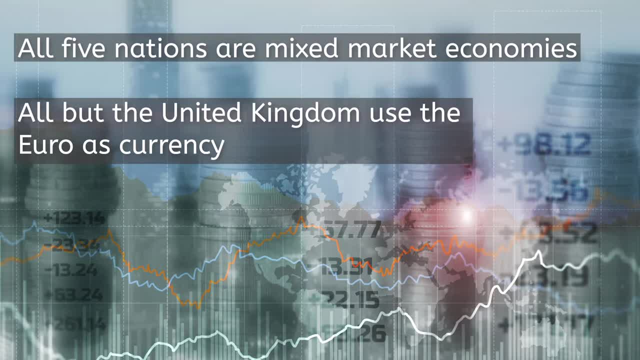 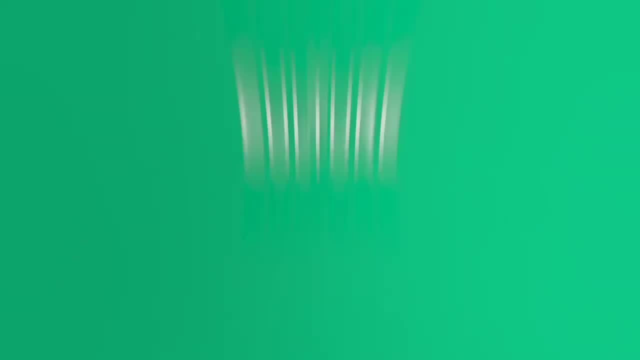 the European Union. Remember, the United Kingdom opted out in 2012.. The United Kingdom opted out in 2020.. They also use the Euro as their national currency, while the UK features the pound sterling Culture. Each of these nations possess cultural icons for which they are famous. 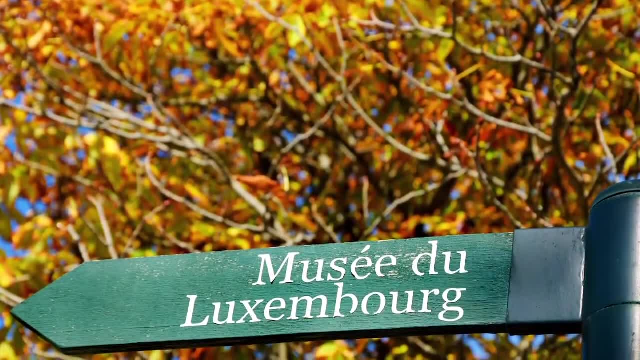 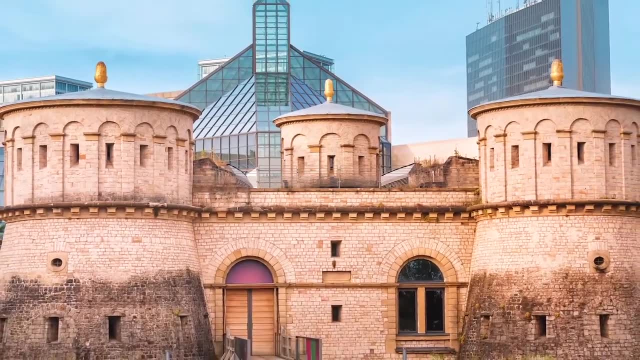 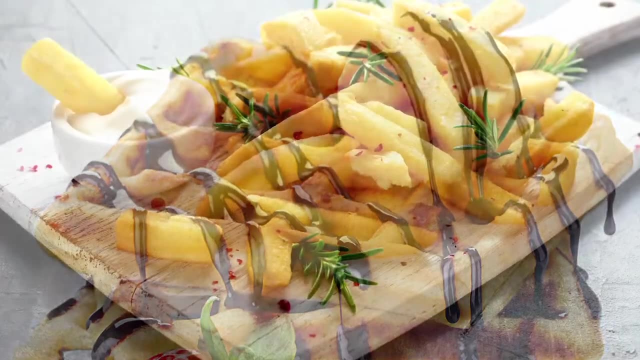 Let's look at a few for each. Luxembourg is noted for its many museums and cultural diversity. In fact, Luxembourg City was the first two-time honoree as the European capital of culture. Belgium is famous for its waffles. Belgium is known for its waffles and chocolate, as well as beer.